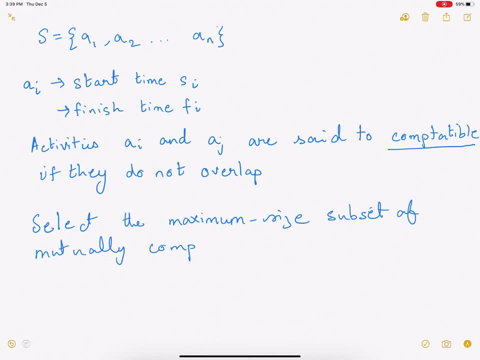 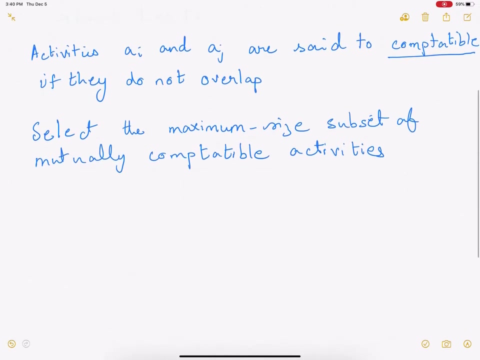 So there are a lot of activities. some of them are not compatible with each other, and your goal is to select the maximum size subset of mutually compatible activities. Okay, so that is the activity selection problem. So to solve this problem, what we'll first do is sort the problems by finish time, That is, we sort. 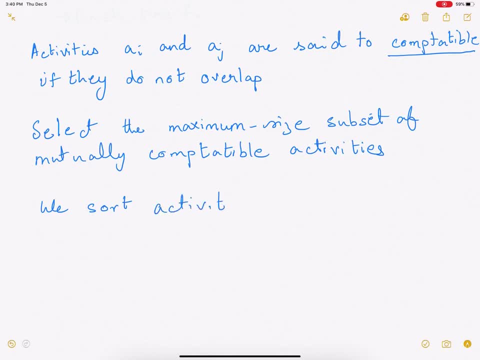 pro activities by increasing finish time. So so we're going to order these activities and what we're going to. so f1, less than equal to f2, less than equal to f3.. So these are n activities and we're just going to sort them out by finish. 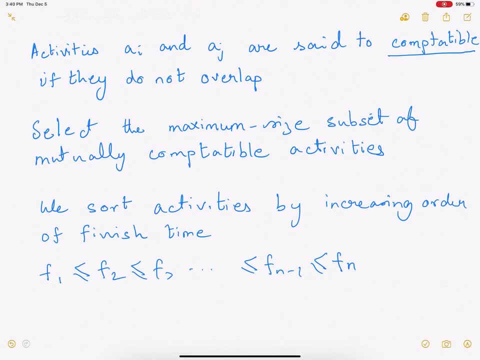 time. So these are n activities, and so fn has the the finish time furthest into the future. f1 is the activity that finishes first. Now, the thing to note is, just because an activity finishes first does not mean that that activity has begun earlier. Okay, so different activities can. 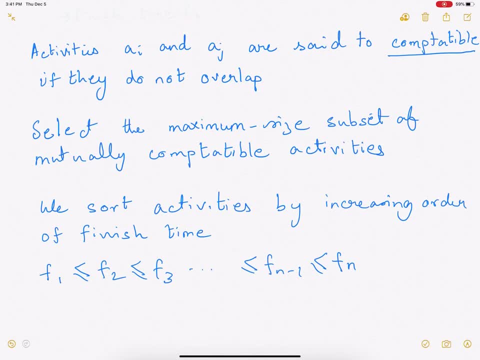 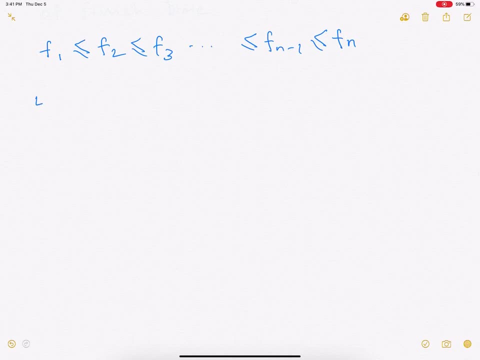 have different duration and they can finish at different points in time. So to understand this, let us first consider an example. So I've in this, in this example, I've sorted all these activities by finish time. so we are going to consider an example where there are 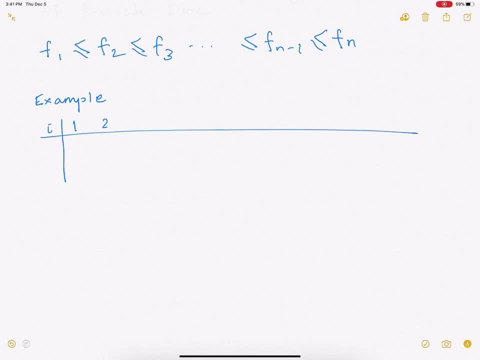 11 activities, so i is the activity: 1, 2, 3, 4, 5, 6, 7, 8, 9, 10, 11. so there are 11 activities. the start times are 1, 3, 0, 5, 3, 5, 6, 8, 8, 2 and 12, so these are the different times at which these 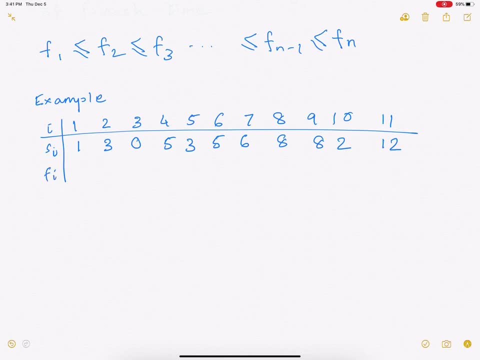 different activities start. now the finish time for these activities is sorted. so these are the finish times of the activities and they're sorted in increasing order. so, as you can see, some activities start earlier but then finish much later. for example activity 10. it starts way early. 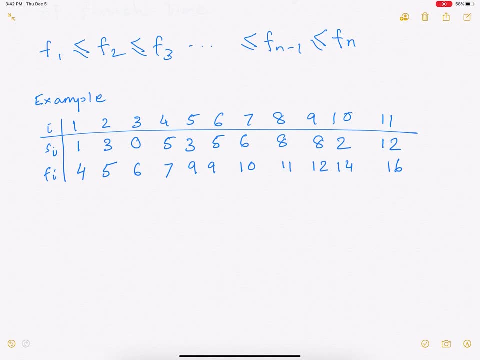 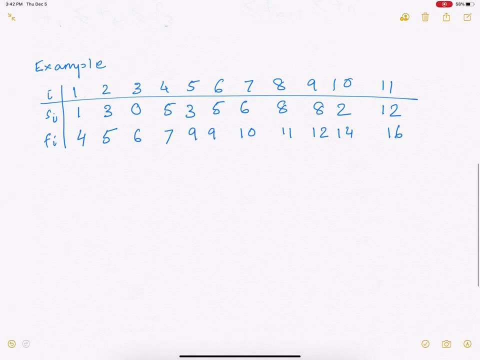 that is at time 2, but it only finishes at 14. so different activities, so different durations, and they start at different times. now let's try to figure out some mutually compatible activities. there's activities that you can do now. the goal is to find out the maximum set. so first let's understand what are mutually compatible. 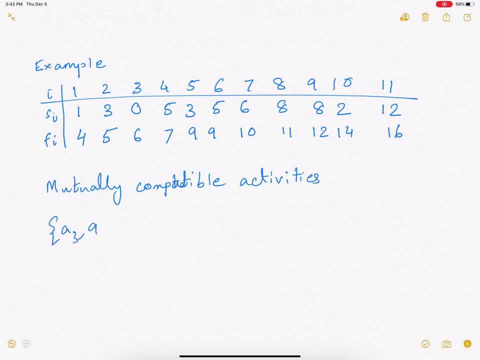 so if you look at a3, a9 and a11, these are mutually compatible. so a3 is: is this one starts at 0, ends at 6, a9 starts at 8, ends at 12 and 11 starts at 6, 12 and ends at 16, so you can do all these three different activities. 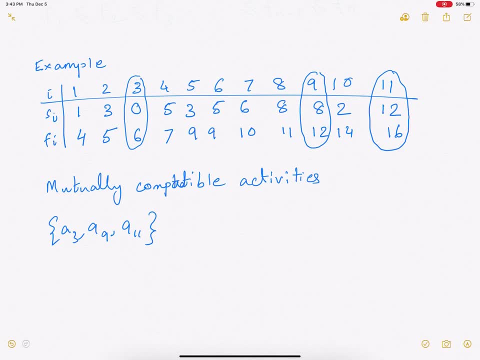 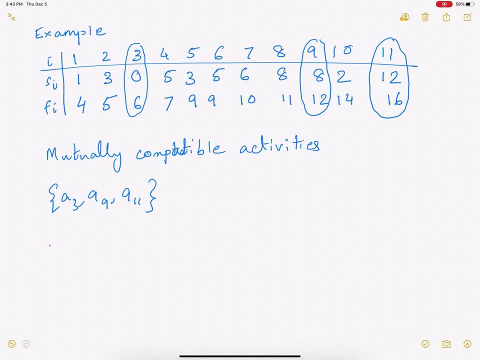 okay, now what is the maximum subset? is this the maximum? the maximum is not. there are activities. there are two maximum subsets: the maximum. so the maximum is the maximum set. so the maximum is the maximum subset of activities. may not be unique, and we'll see this for this example. so there are two. 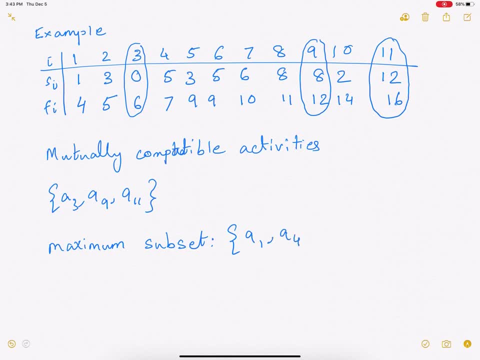 such things. one is a1, a4, a8 and a9. this is one. these are four activities that you can do. another one is a2, a4, a9 and a11. there may be others as well. i'm just mentioning these two, so now let's erase. 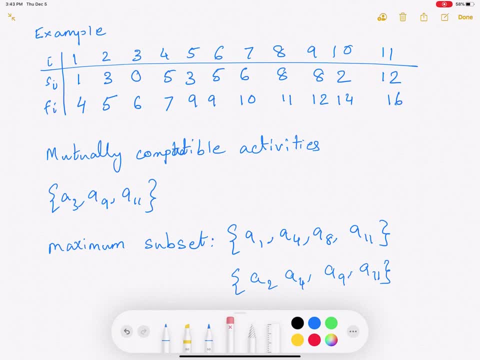 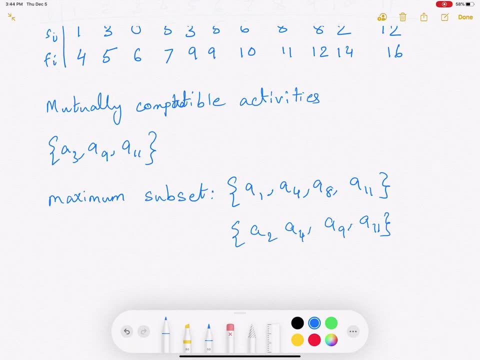 these. so what we have are mute maximum subsets. so what we can see is there are multiple options here. some of them are not as large as others, and even the maximum there can be multiple options, so the solution to this problem is any one of these two. any one of these two is a solution. 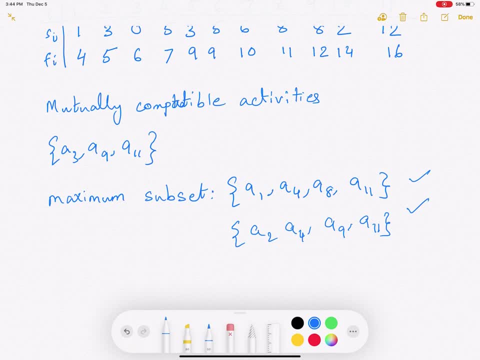 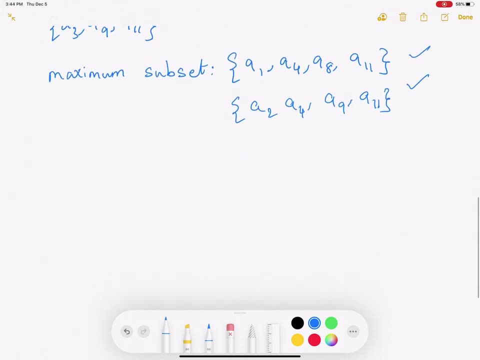 to this problem. so how do we get the largest set of mutually compatible activities? so to do that, we'll take a greedy approach. so there is a greedy algorithm now. for those of you who are listening to greedy algorithms for the first time, a greedy algorithm is an algorithm which makes a 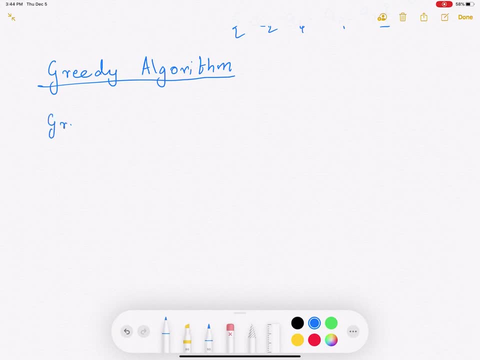 greedy choice. that is, it chooses something that looks best at present and it keeps repeating that choice till there are no other options left. okay, now the greedy choice here is one greedy choice. there could be others as well. this is what we are going to choose and this will give us the optimal solution. choose activities with earliest finish time. 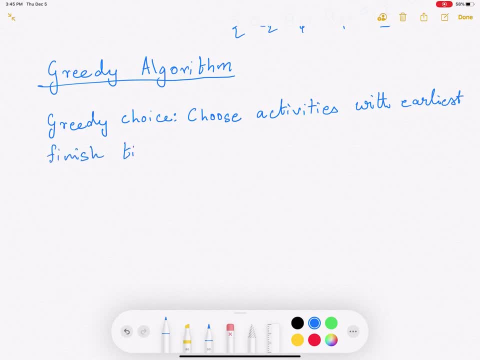 so you keep choosing activities with earliest finish time. of course, you have to make sure that the activities that you choose are mutually compatible. now we will denote by u this set of these of sort of sorted activities, okay, by finish time, and we'll see why this is. 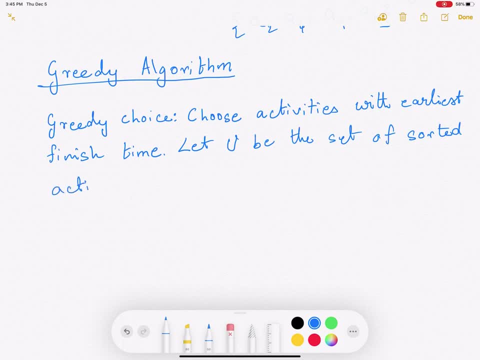 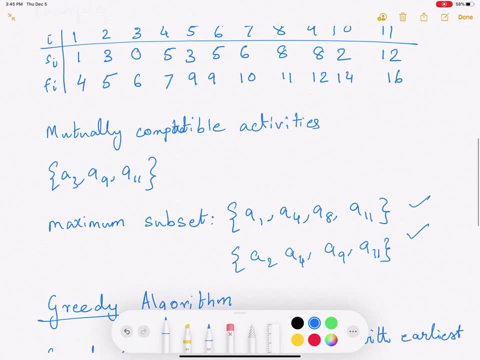 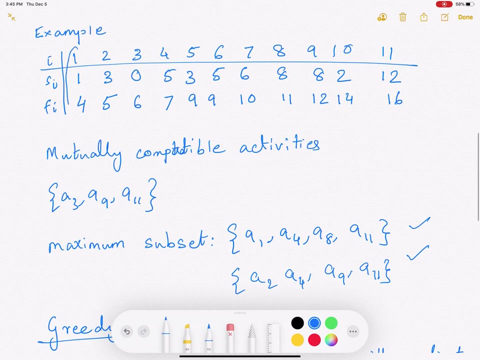 needed when we look at the pseudocode. so if we follow this logic for this problem, we'll first pick a1, so i'll first pick a1, so first pick a1. now we cannot pick a2, or a3 for that matter. we cannot pick a5, because these are all activities that will are not compatible. 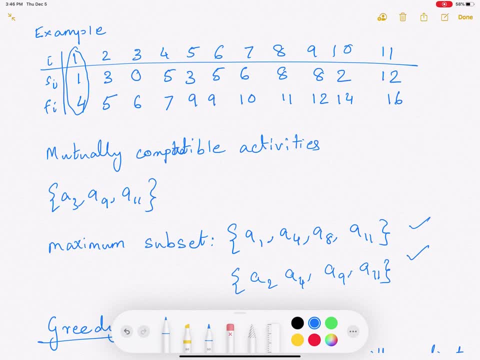 with a1. so you first pick this one, then what you're going to do is you're going to pick the next activity. you keep going down this line. okay, two cannot be picked because it's not compatible. three cannot be picked because it's not go to four. yes, four cannot can be picked, it's compatible. 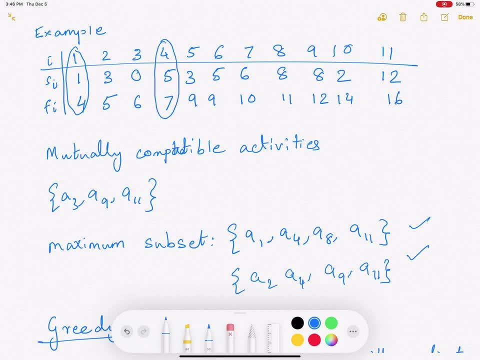 so you pick four, then you go here. that's not compatible. this one's not compatible. you go here. this one's not compatible. this one- yeah, it's compatible because it starts at eight and a4 ends at seven and then nine- is not compatible with eight because it's only ends at eleven. 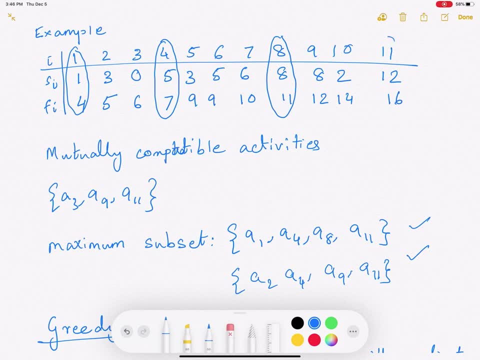 ten is also not compatible, and then eleven seems to be compatible. so go here so you will actually get this one, this one- i'm going to put two more ticks here- that particular solution using the greedy algorithm that i just described. so that's how. that's a greedy algorithm for the activity selection problem. so how do you go about? 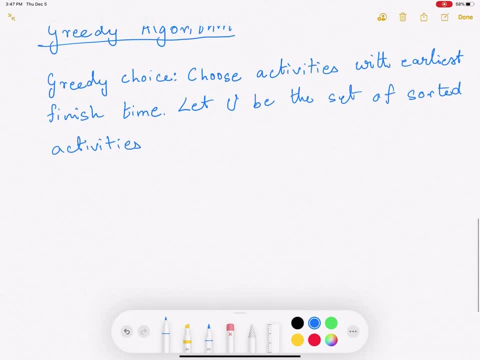 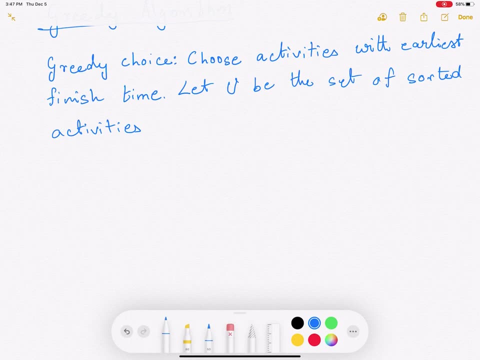 implementing this. so it's a pretty simple algorithm. i'll just talk about the pseudocode next. so you have sorted all activities by by finish time and you're going to pick them off. so the greedy algorithm- so i'm just going to write it- greedy select- this is the algorithm and it's going to take in the start and finish times of all these. 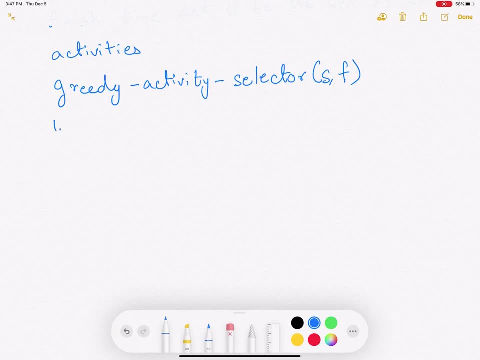 of all these activities. so you're first going to have n, which is basically the length of all these, all the any of these two arrays, because this is the number of activities. start off by picking a1, the first activity, the sorted list then, and find k equals one. what you're going to do is you're going to loop. 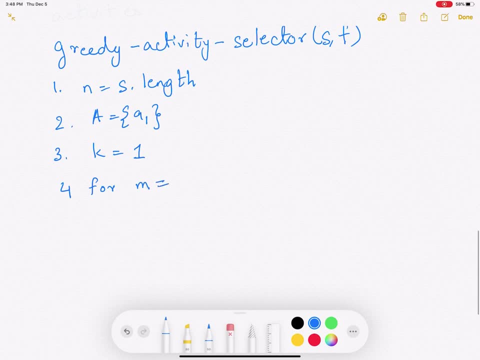 through the remaining activities to see if they can be picked. okay, now, if s m, the start time, is greater than equal to fk, the finish time of the activity that has currently been picked, then you will actually add this activity to your list. so initially, if you notice, 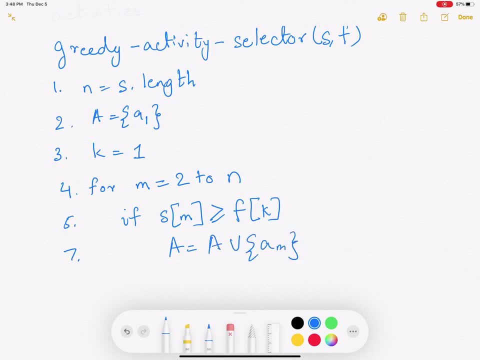 k is one. so you always pick the first activity in this approach and then what you do is you go through the remaining activities, two to n, and see if, when, which activity overtakes the finish time of the first activity Once you get that Activity. 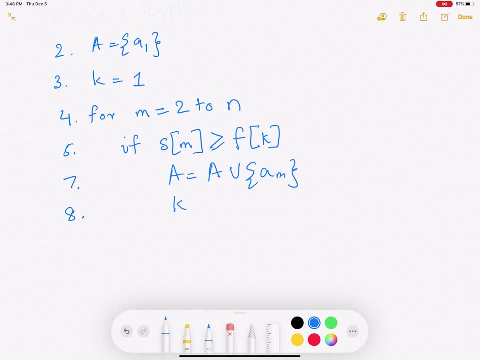 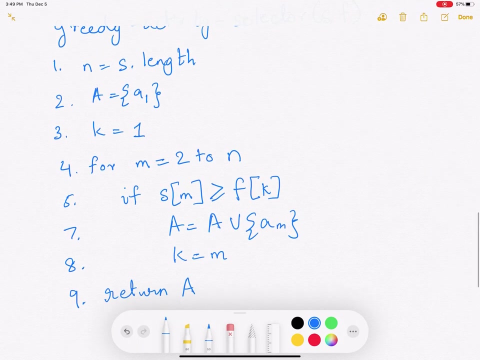 What you're going to do is you're going to update K. Okay, so update k, and then k will be m, so you then go on. so you're basically going to go through this entire set of activities one, and once you've done that, you are going to get the maximum sized activity subset. so this is our greedy algorithm for red.